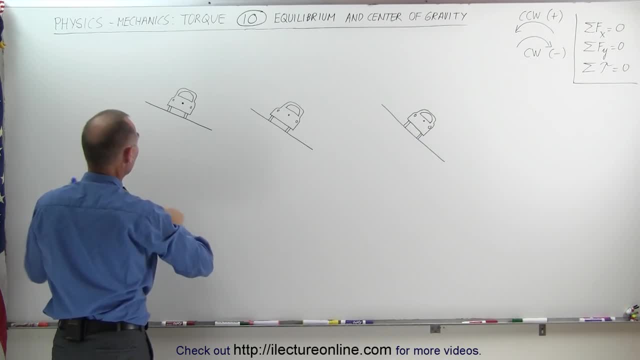 the car. If we now draw a arrow from that point directly downward, you can see the. this is where the total weight of the car is acting, and notice that the line of action of that force that represents the total weight of the car acting at the center of gravity is to the left. 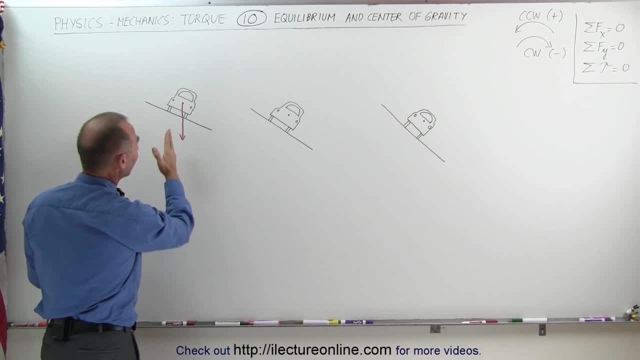 side of the outside support of the wheel. As long as that line is to the left side of that wheel, the car will stay there and will not tip over. Also, another way of thinking about it is that the weight is distributed across the two tires. if it's angled like this, more the weight is. 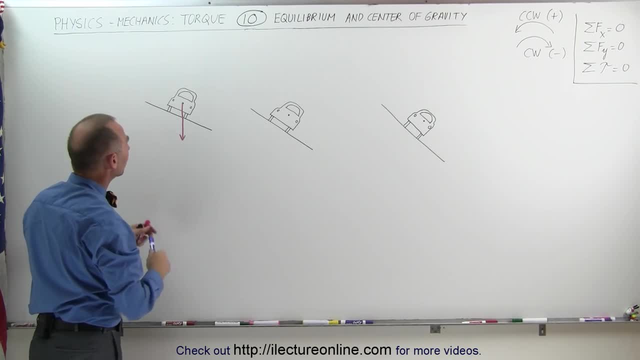 is being supported by this tire than by this tire, and if you use a different color, you can see that the vast majority of the weight is supported by this tire. a small amount of weight is supported by this tire, but you can see that. if you then put a pivot point right there. 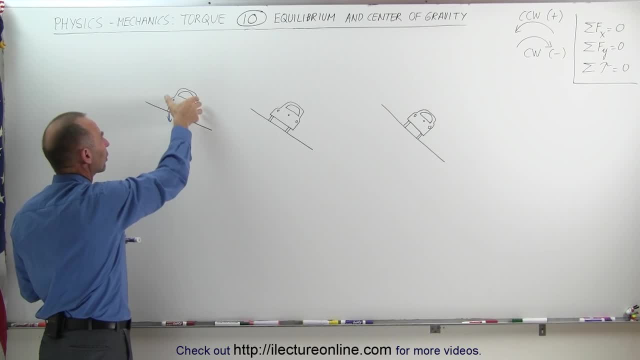 then you sum up all the torques about this point, you can see that there's a net torque causing a counterclockwise direction on the car, preventing it from tipping over. Now, if you look at the data for the base model, as you look at, this currentsorrystock number that we're dealing with is about 97%. 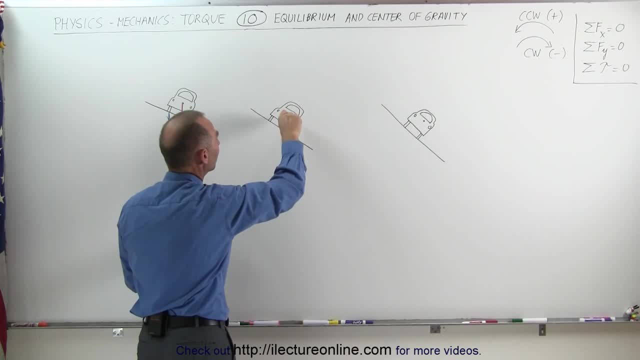 next picture. here you draw an arrow from the center of gravity of the car straight down. Notice it goes right through the support on the right. At this point you can see that all of the weight is supported by the right tire and none of the weight is supported by the left tire. If we use 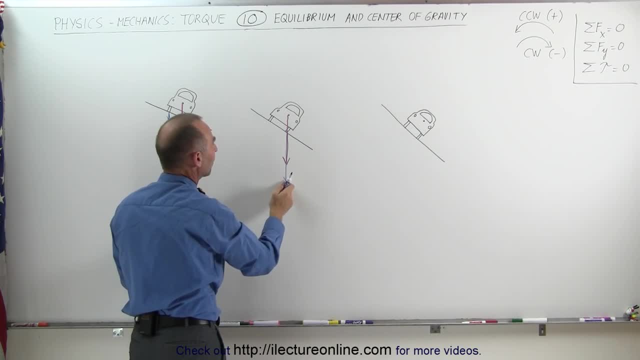 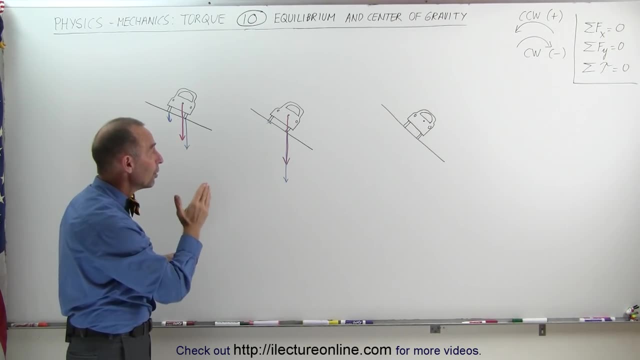 blue to indicate that you can see that all of the weight is supported by the right tire and no weight here is supported by the left tire. At that point the car is just at the point of tipping over Any small amount of force to get it going, or any small amount of wind or small amount of movement. 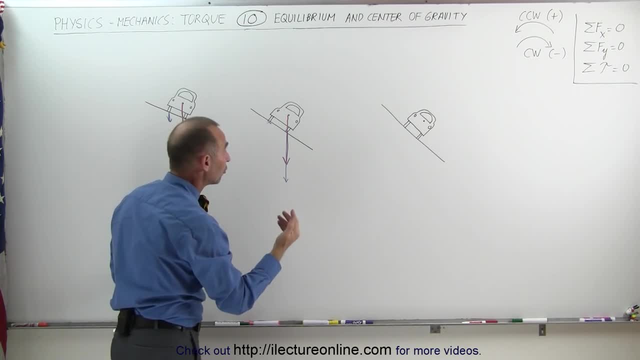 there could cause the car to tip over. If you want to sum up the torques relative to this pivot point right here, notice there is no force on this tire causing no counterclockwise torque, and so you can see then that this car is just teetering on the edge of falling over. Now, when we come to this, 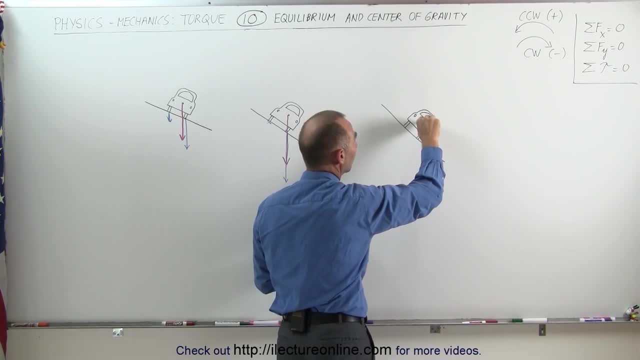 picture right here and we draw a line, an arrow, from the center of gravity straight down. you can see that if all the force, all the weight is supported by the left tire, the car is just at the center of gravity and the center of gravity is just down. it passes to the right, of the rightmost. 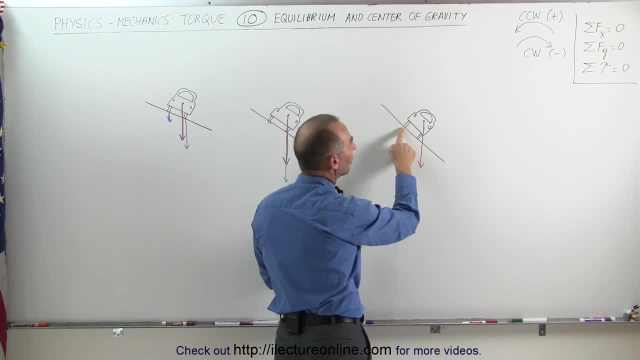 tire, which means that no weight is being supported by this tire. Not all of the weight is supported by this tire, because at this point the center of gravity is acting to the right of the tire. and if we then sum up all the torques about this pivot point right here, you can see that if we let this 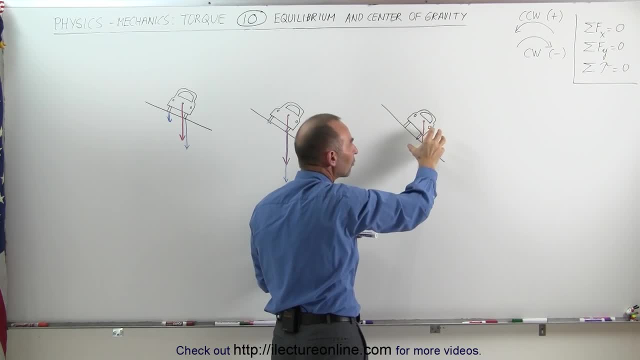 be the sole force. the center of gravity is acting to the right of the tire. the center of gravity is acting to the right of the tire and if we let this be the sole force acting on it, it will cause a clockwise torque on the tire, on the car. There's no counterbalance in the opposite direction, because 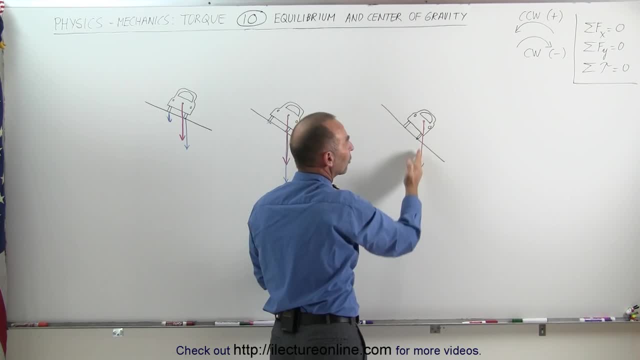 any force supported by this tire would go right through the center, right through the point of rotation. On the left side of the tire there's no weight at all being supported by this tire, so the car would simply fall over. It all comes down to the location of the center. 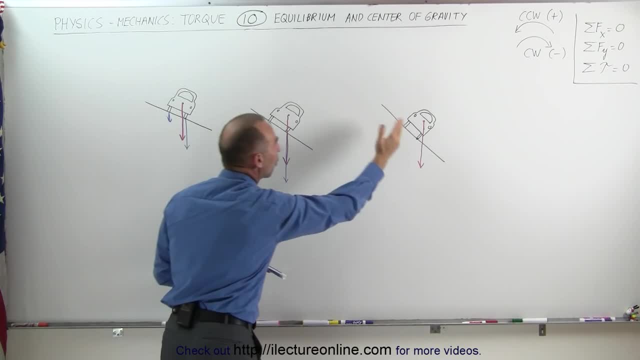 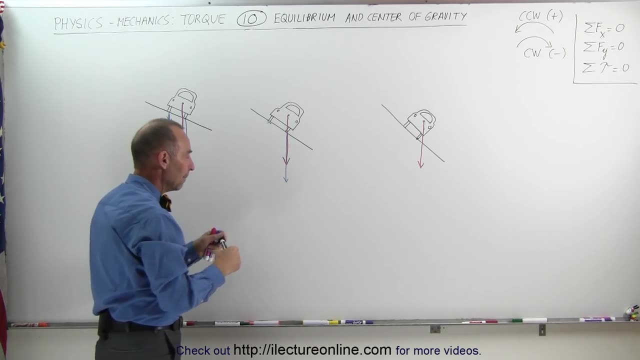 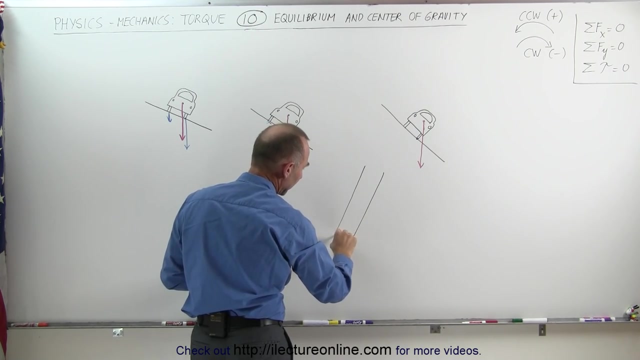 of gravity and where it's relative to the support. Another famous object that most people know about is the Tower of Pisa in Italy. It looks kind of like this: It's leaning quite a bit, the leaning tower, and there's maybe some structures here where people can stand around and 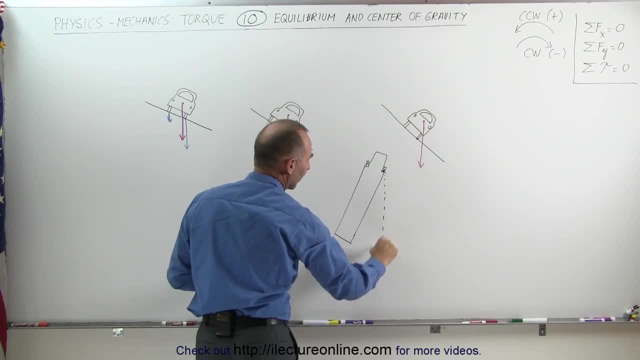 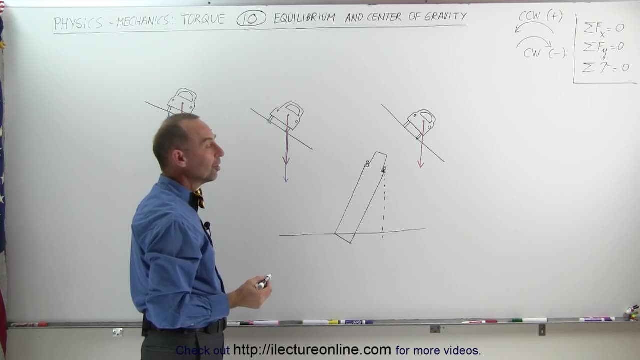 I guess we have the famous Galileo, the dropping object from the tower to see what was going on there. But now let's draw the line this way, And the whole question is: where is the center of center of gravity relative to the rightmost support of the tower? If the center of gravity 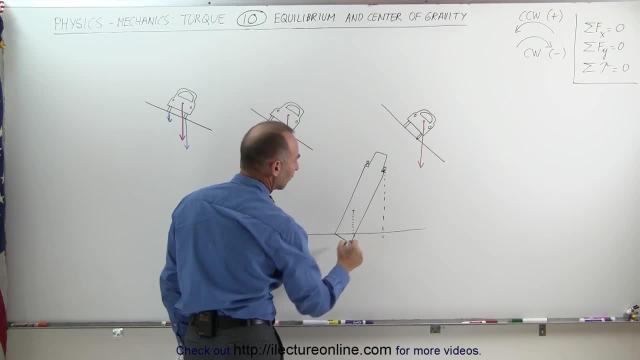 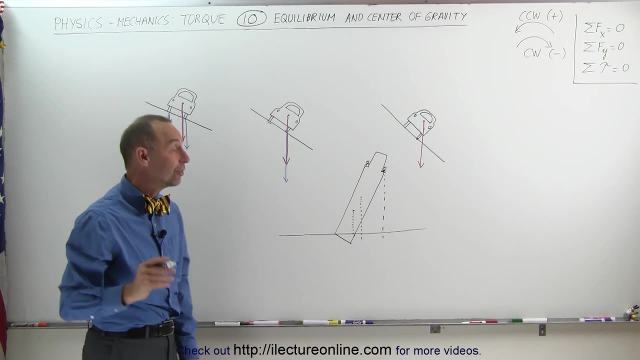 is right here, then you can see that the tower will not fall over. But if the center of gravity is right here, then you can see that the tower will fall over. So what have they done to keep the tower from falling over? Well, one of the things that they've done if they stacked 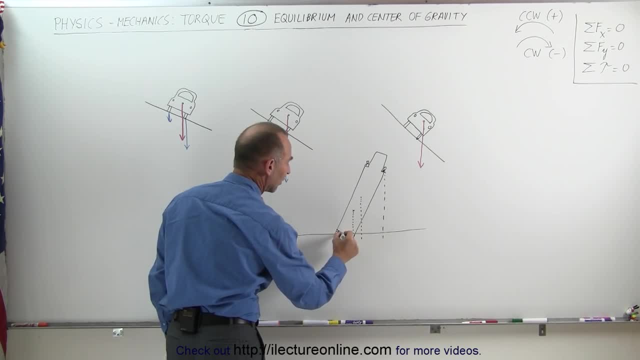 up a whole bunch of big lead blocks right here. of course, lead is very heavy, so they stacked up a bunch of lead blocks on this side of the tower to try and move the center of gravity to the left in such a way that it would stay to the left side of the outermost. 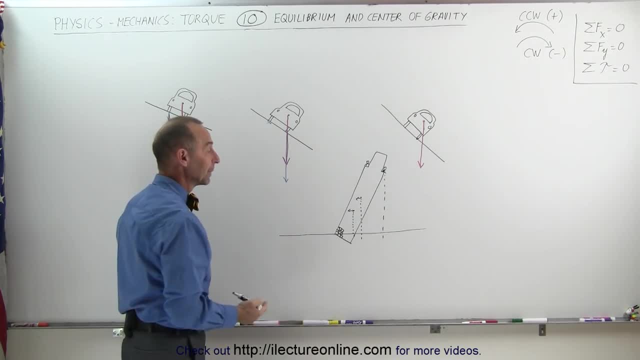 support of the tower, hopefully keeping the tower from falling over. I don't know if they'll be able to keep the tower from falling over in the future, but at this point they've been able to do so. They've tried all kinds of things to support the site. Of course I've